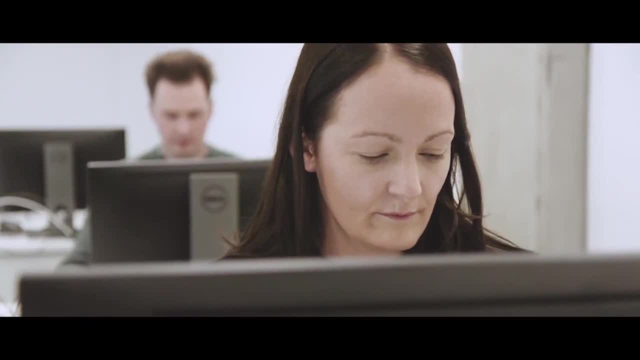 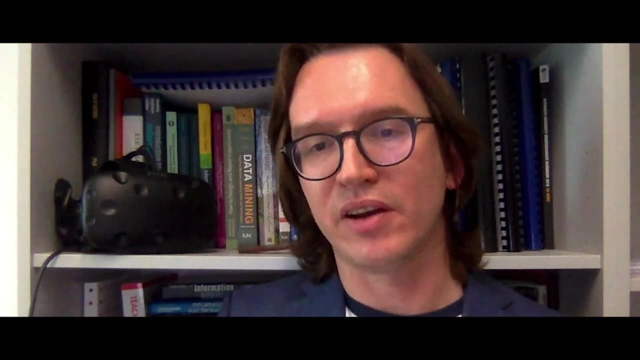 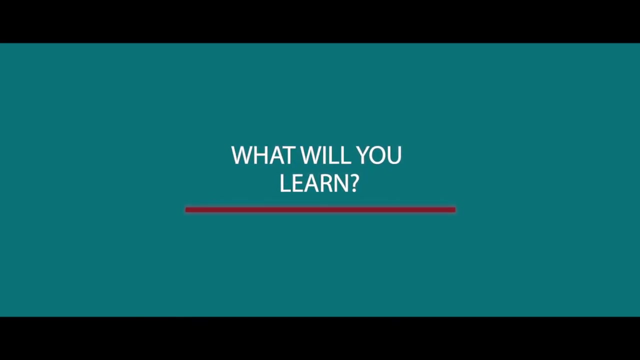 interfaces and what we do. It helps us making decisions. So we have a component of data science and visualization in there And we connect that with a wide range of technology: mobile devices, virtual augmented reality. We have a wide range of practical subjects that include such things. 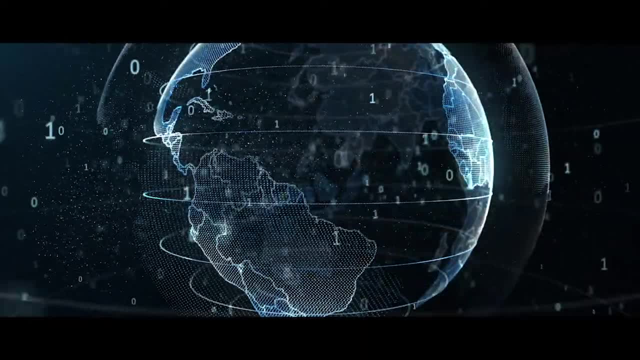 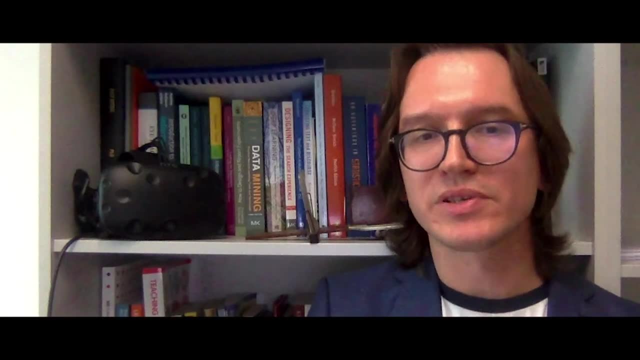 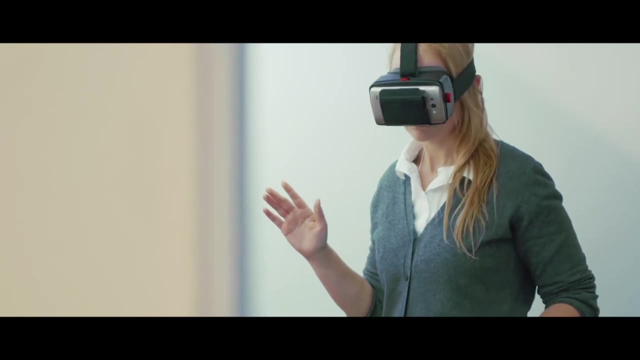 as web development and interaction design, So you learn about web frameworks, JavaScript, HTML. Mobile development, so mobile application development and mobile platforms. Multimedia technology, so everything about images, video, audio, virtual reality, 3D environments. We have. 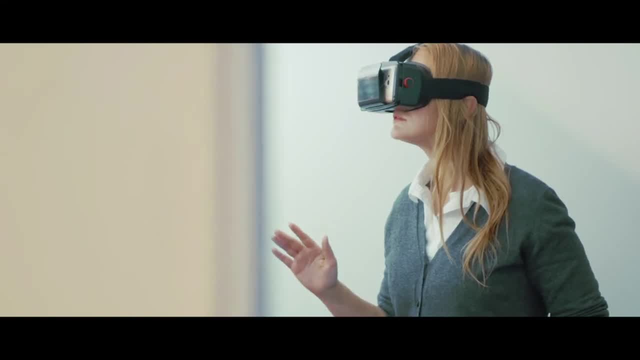 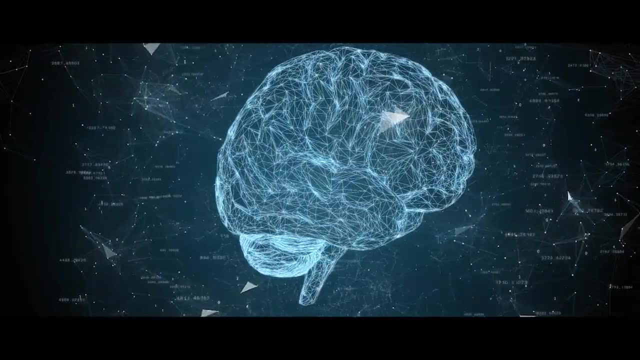 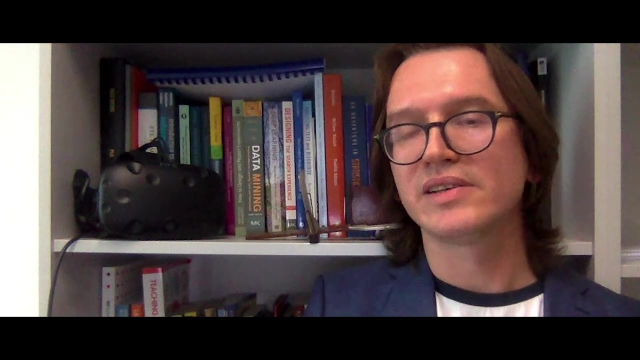 a specific module about virtual reality, augmented reality and mixed reality. We cover machine learning, artificial intelligence and data analytics, and also ethical questions. Maynooth University has 20 years of experience in these areas, including HCI, software development and data analytics- AI- machine learning. We also collaborate. 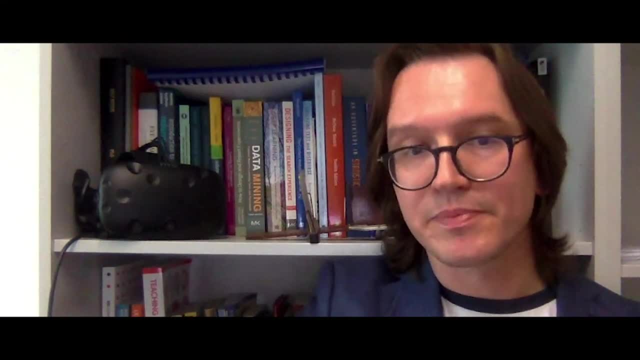 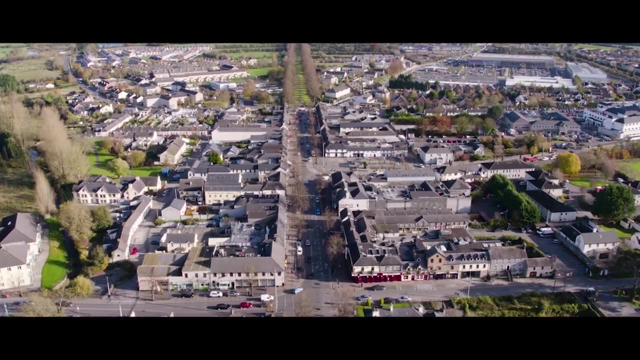 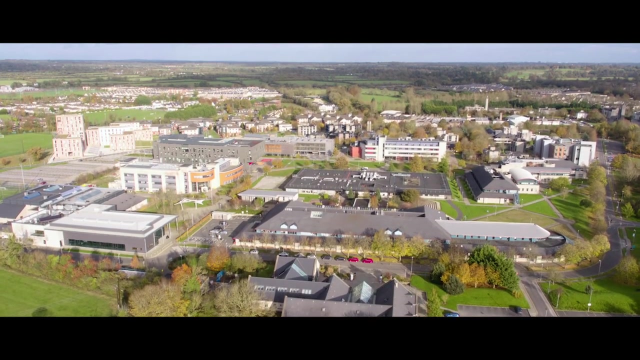 with the philosophy department on the questions of ethics. And Maynooth University itself lies at the center of a very vibrant town with a very large student population and a wonderful and beautiful campus. This is a one-year full-time program funded by the Human Capital Initiative. 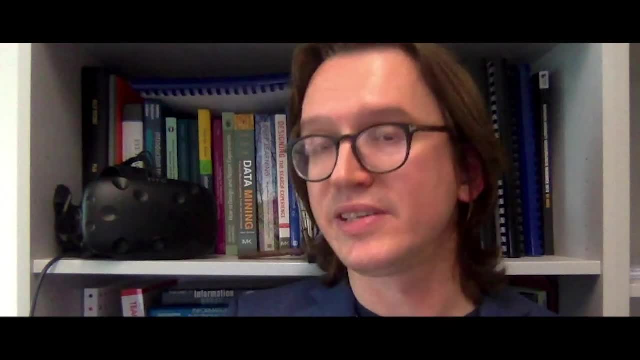 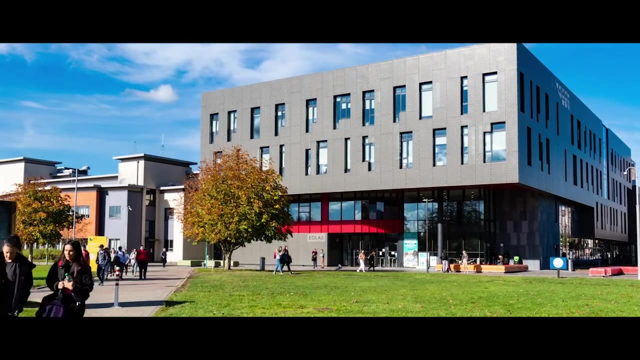 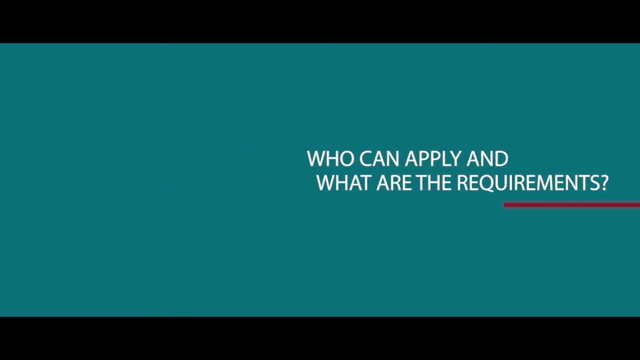 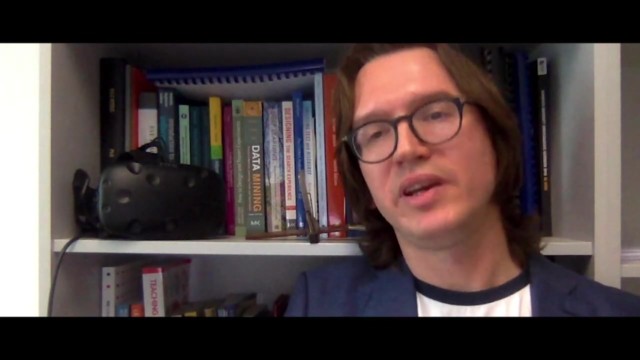 and it is funded to prepare graduates to design and to develop and to evaluate user interfaces with modern applications and modern technology. You need to have a completed three-year undergraduate degree, but it does not have to be in computer science. You can have a wide range of backgrounds for that degree, including computing. 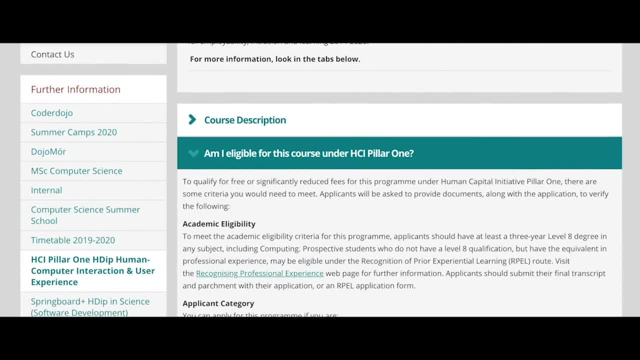 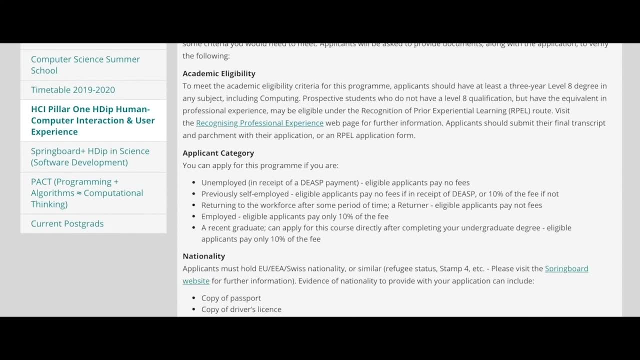 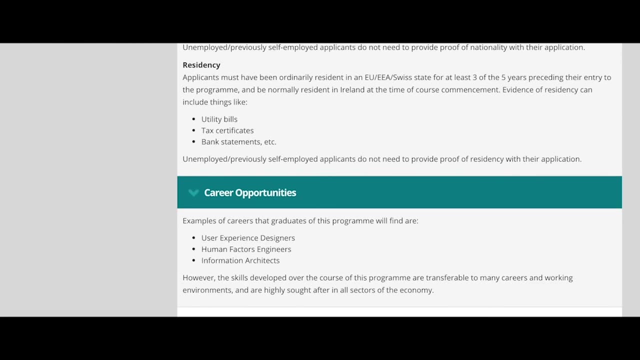 You can also enter the program through the recognition of prior experiential learning. It is open for unemployed, for the self-employed or formerly self-employed, the returners. when you're a recent graduate, you can apply for this program and you can also apply when you're employed and you want to upscale.